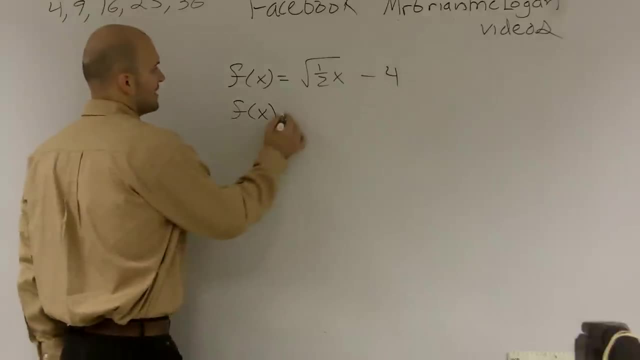 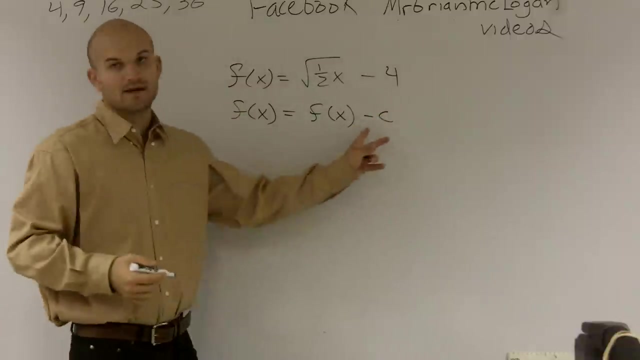 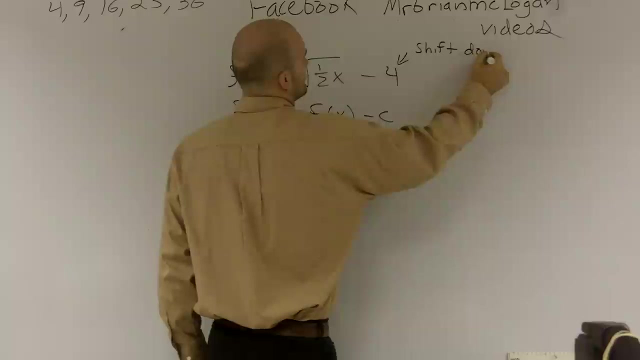 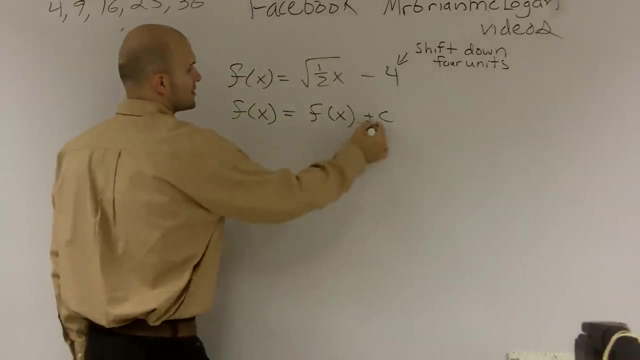 and if we do anything to that f of x, if we do a minus, you know c. what that means is that's going to be a vertical shift downward. So we're actually going to be shifting our graph down four, Four units. Alright, So that was always like your plus or minus, Remember. 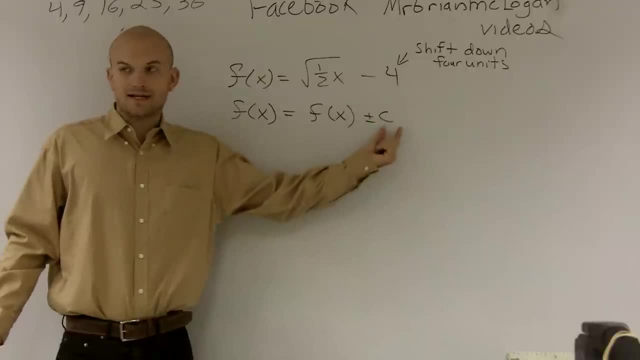 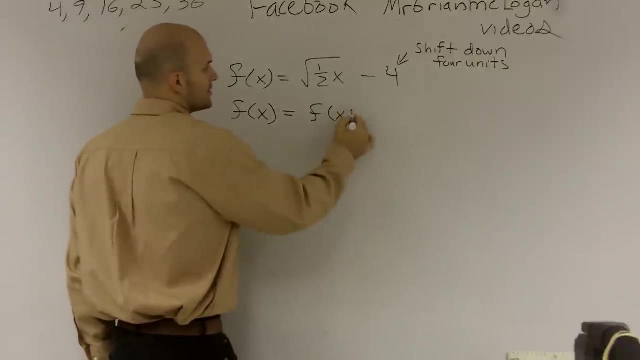 whenever you have your function and you're adding or subtracting any kind of number, that's going to tell you if you're shifting up or down And if we were to do plus or minus inside of the function, that's going to tell us to shift our graph left or right And remember. 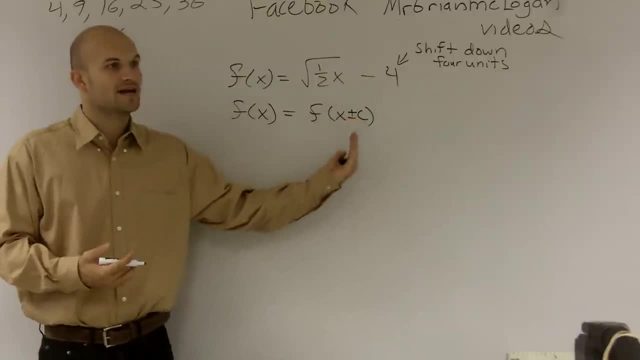 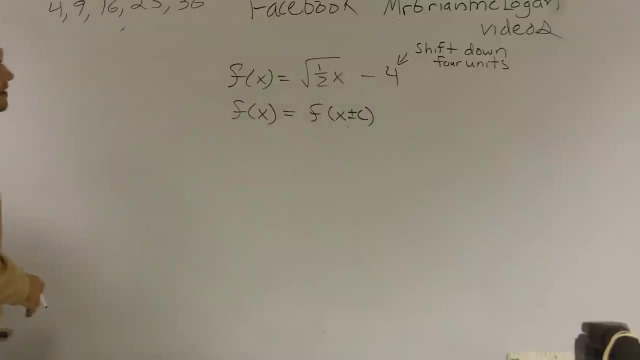 for right now, that's always going to be the opposite, right. If it's positive, it actually means you're going to be shifting to the left, and if that's a negative c, you're actually going to shift it to the right. So let's look at our next kind of transformation. This is 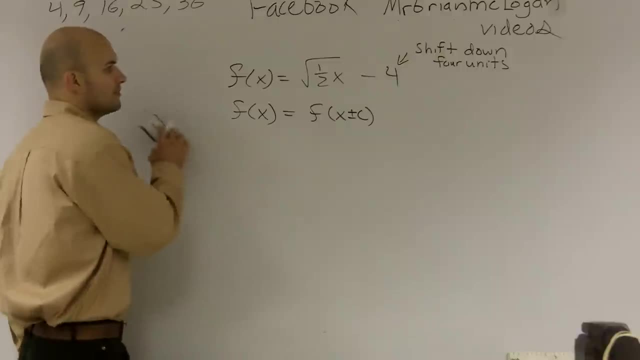 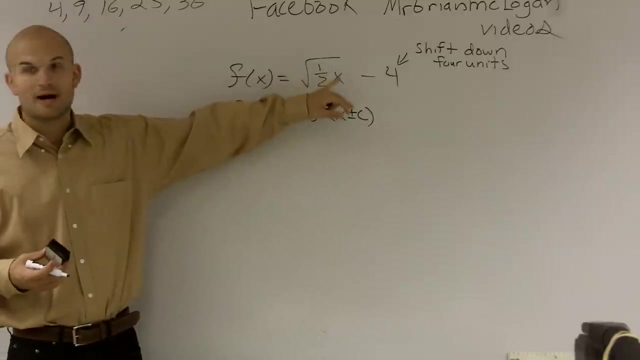 going to be a non-rigid transformation, And what I mean by non-rigid is it's actually going to affect the shape of the graph. So what we look at is we have a number that's now multiplied by our x coordinate or x value. So there's a couple things we need to look. 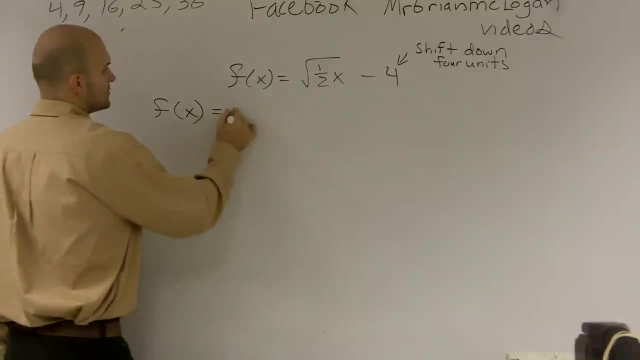 at. If we have f of x equals c times f of x. what this is going to do is this is going to give us a vertical: either shrink or stretch. It's actually going to change the points. Now, if you guys remember when we were talking about functions, if we have a function and 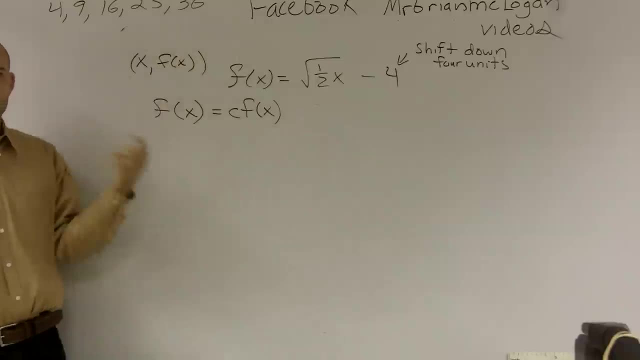 we look at the graph, we have two coordinates: It has an x and it has an f of x, Very similar to our x and y. But we're going to be using our f of x as our output value. So when you're. 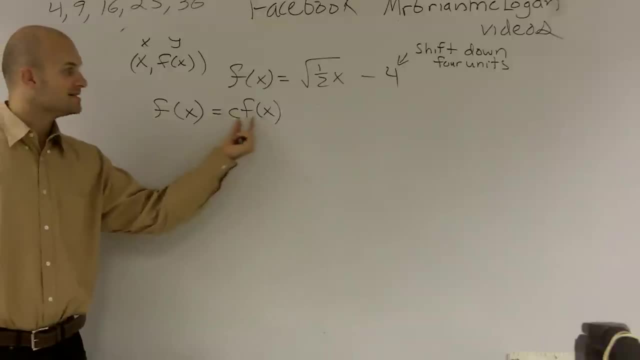 looking at this, if you're saying, all right, now I'm going to multiply a constant times my output value, what's going to change that output value? So when you're looking at the graph, I don't even know what the graph looks like at this point. you know that now, if I'm 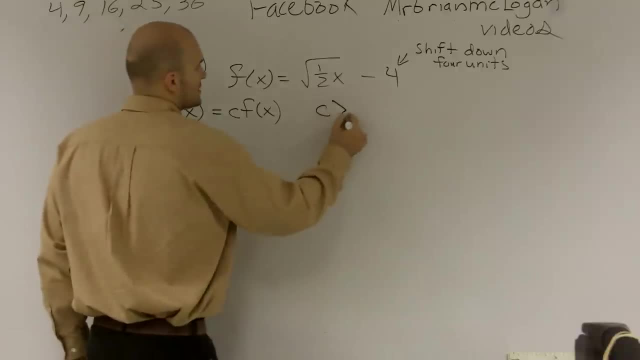 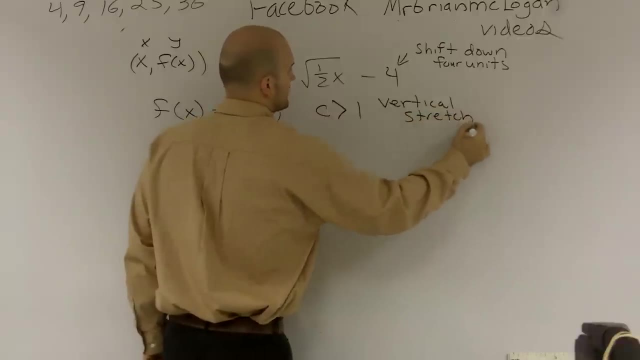 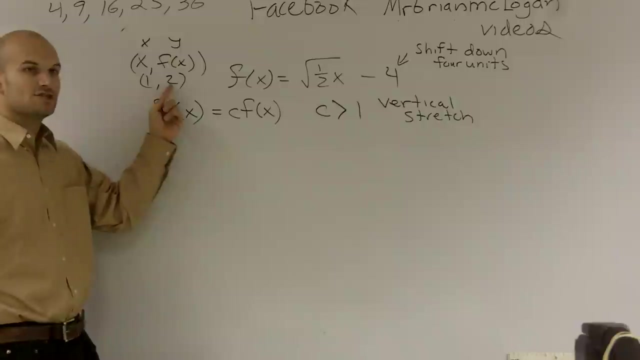 multiplying it by a number, if that number is greater than 1, it's going to be a negative 1, it's going to be a vertical stretch. So if I multiply by 2, think about, let's say, your point is 1 comma 2.. Well, if I multiply 2 times 2, now it's going to be 1 comma 4.. 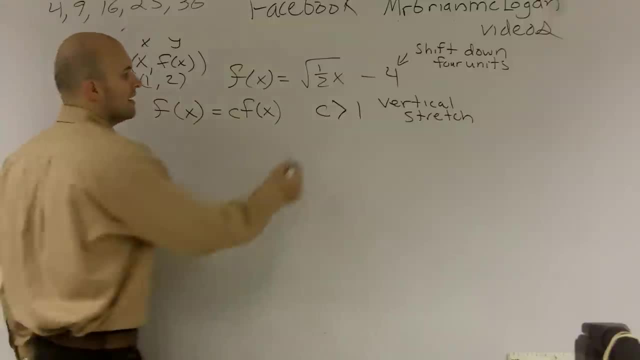 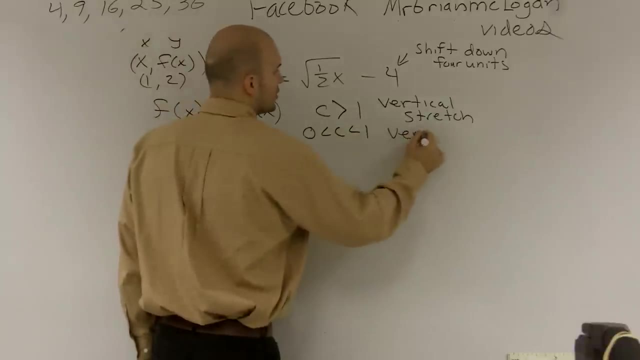 You're stretching it. Whatever you multiply by, it's just going to be your multiplier. And then if c is less than or equal to 1, it's going to be a vertical shrink. So if I multiply by 2, I'm going to be 1 comma 4.. So I'm going to be a vertical shrink. 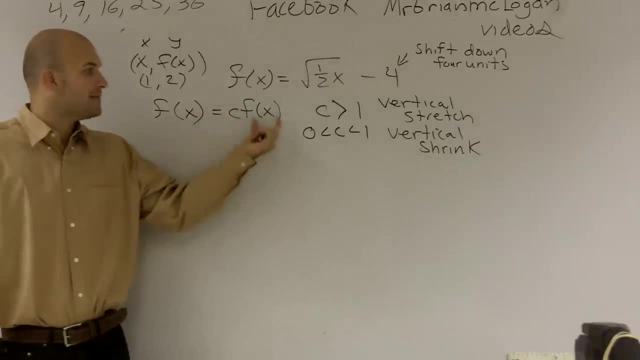 So you guys have to understand: when I'm multiplying a constant by my function, that is going to change vertically the points. It's actually going to stretch or shrink your y coordinates or your output coordinates. Then there's another kind of stretch we have going on which is: 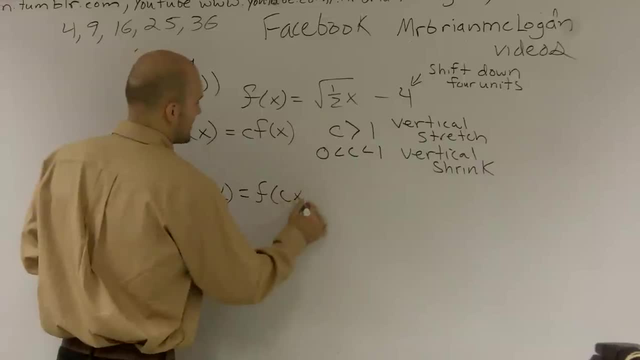 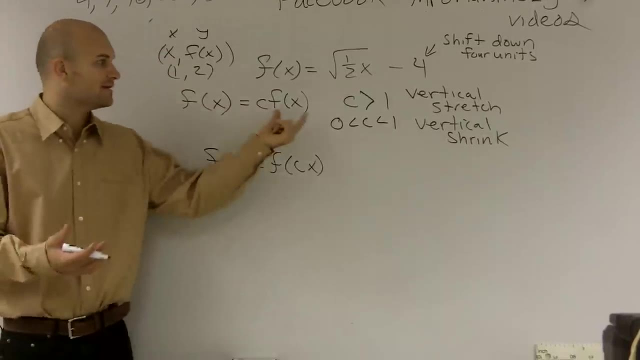 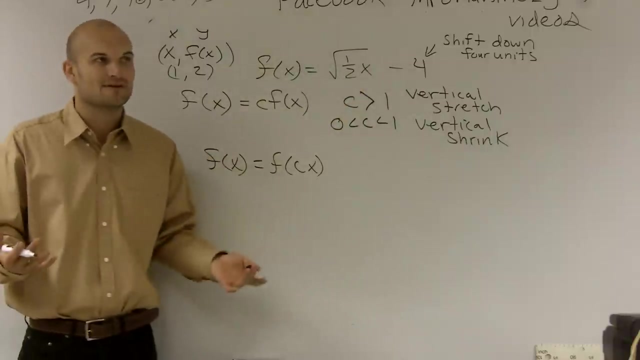 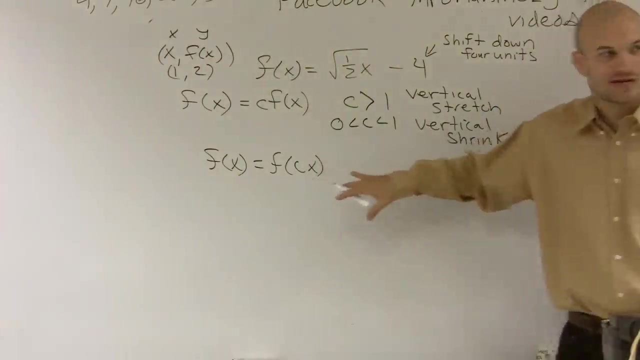 f of x equals f of c of x. So now this is actually affecting the input values. So what do you think? So when it affects the output values, it's a vertical. When it affects the input values, it's now going to stretch it horizontally, And kind of like how, when you did your horizontal 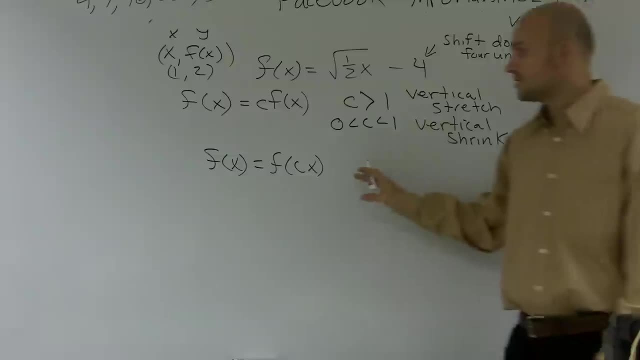 shifts left and right. this is going to be the opposite as well. So when I'm looking at this diagram, when I'm going to do my horizontal shift to expressed from 0, I'm going to ask now if I multiply y right past y. The answer is a bit of a% or a very difficult answer, And it's actually a good idea to divide by your 말�ing. you should weight the y output values on top of your woof object, And what that means is you ain't go into space And you're going to do your matrix. 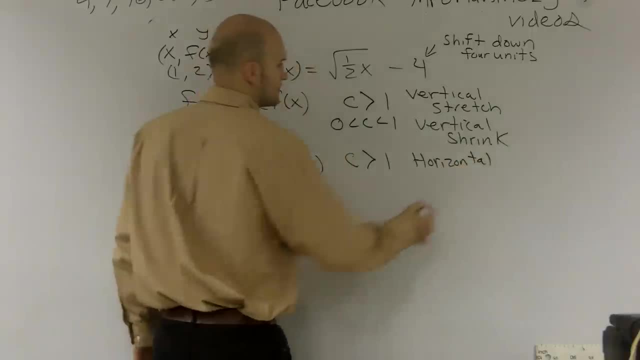 in way over here, in the perspective Which is my есте be, at least this time, You're games And we're going to use x minus y for both of your yaptions, And if c is greater than 1, that's actually going to be a horizontal shrink. 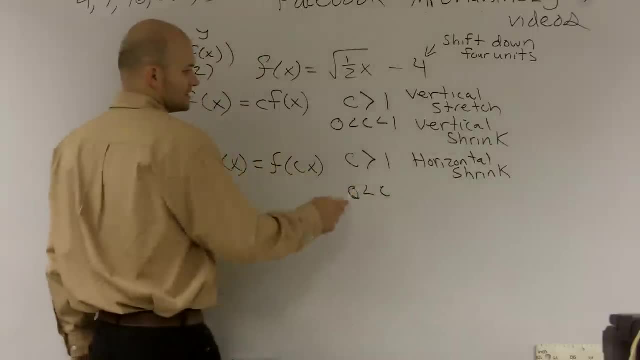 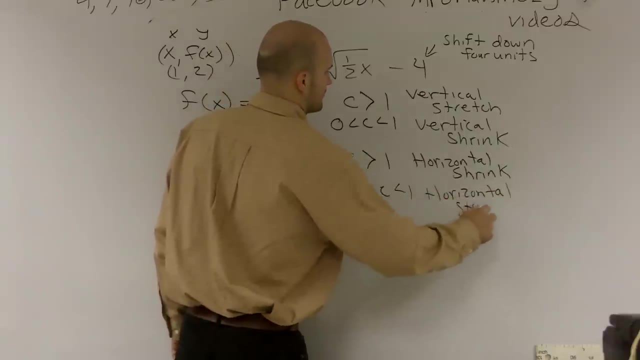 And if c is less than- I'm sorry, Zero C is less, C is greater than 0, less than 1.. That's going to be a horizontal stretch. that's going to be a horizontal stretch, All right. so you guys really got. 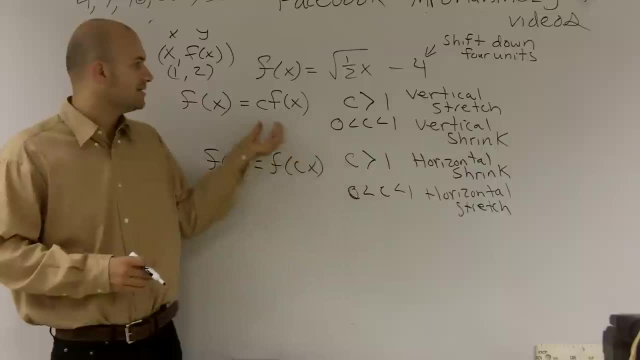 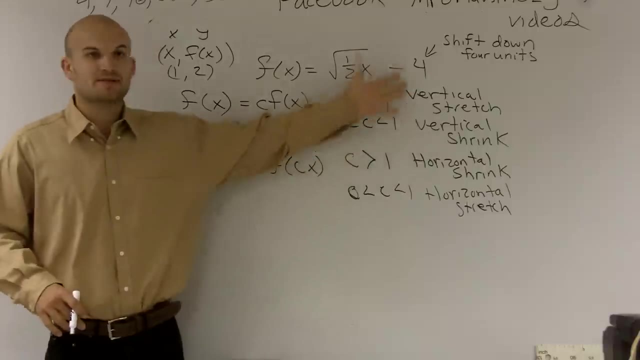 to make sure you remember just what's happening And the easiest way I like to always think about it: just look at what is your c doing. If it's multiplied by your function or your output value, then it's going to be something doing with the vertical stretch. 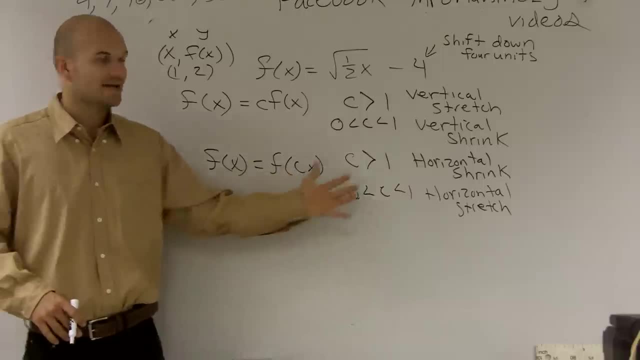 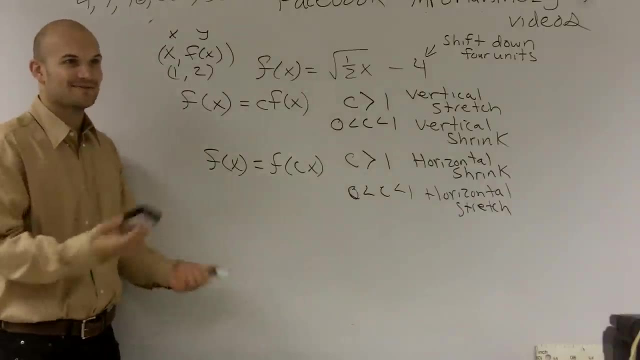 or shrink, And if you're multiplying it by your input value or your x, it's going to be doing something to the horizontal. So let's actually look at the graph. Hope you guys can all take a look at this online, so then I don't have to worry about keeping it up here. 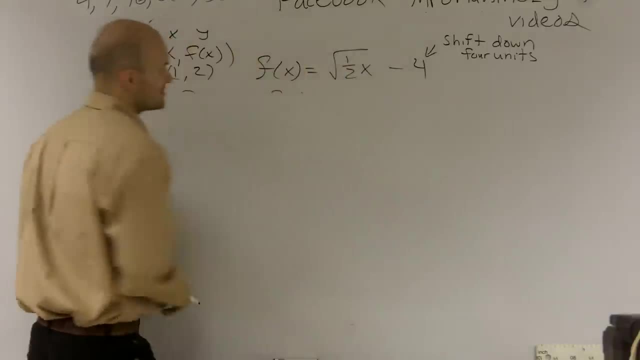 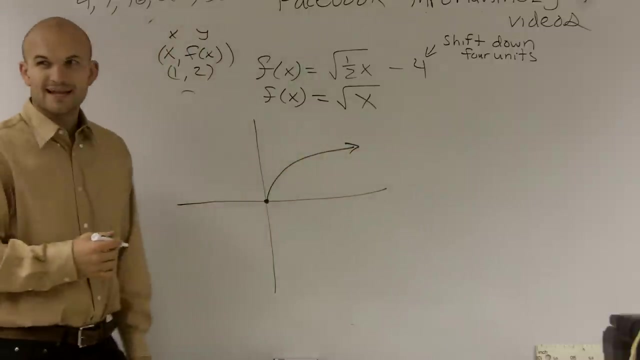 So I'll just erase it. Now let's look at the paragraph. The paragraph is your root function, square root of x. So hopefully at this time, we should now have a rough sketch of what this looks like And let's just pick a point that we want to use. 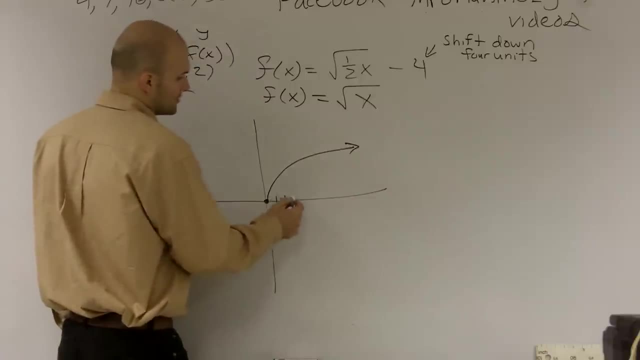 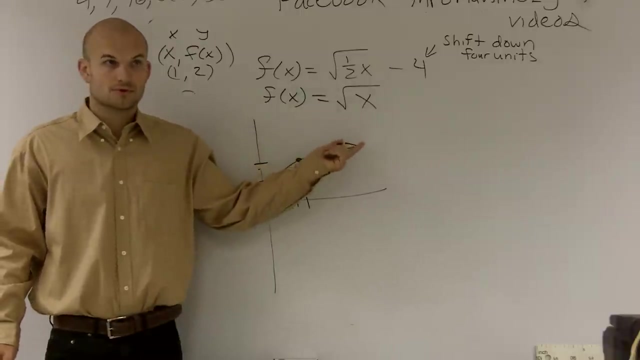 Let's pick the point 4.. 1,, 2, 3. 4. And we know that 4,, 4, 2. Right, Because the square root of 4 gives you 2.. Correct, Right. 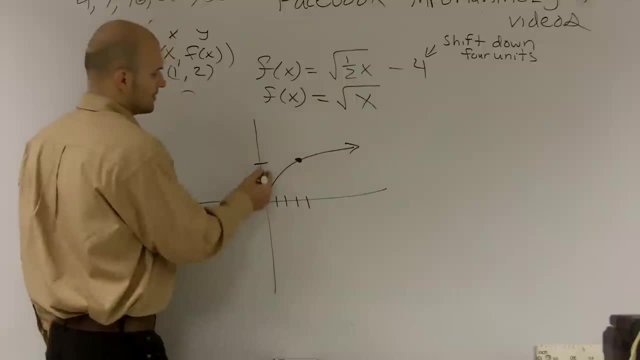 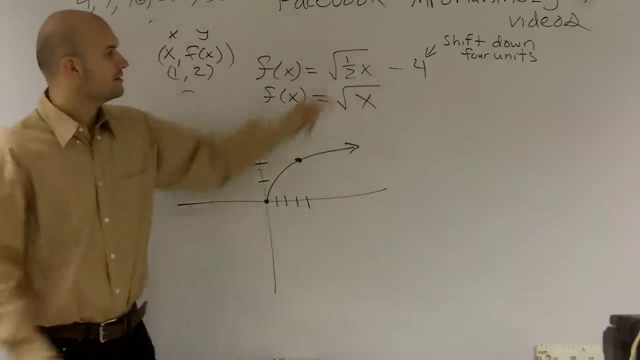 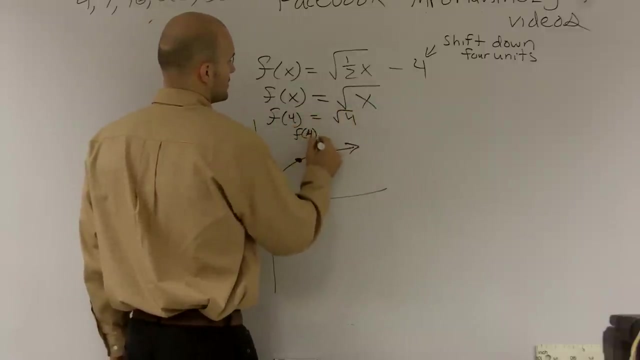 Well, how about let's say: now we plug in, let's try to find this new graph, And if I plug in 4. It's just right here. So if I do f of 4, square root of 4, f of 4 equals 2.. 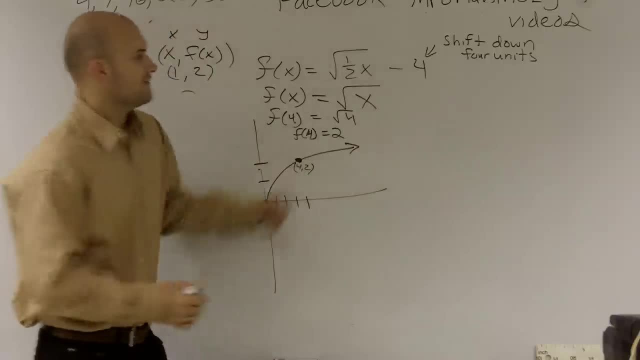 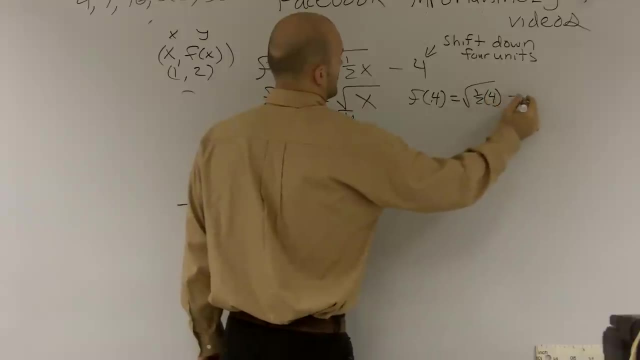 OK, That's what we point, That's 4, 2.. Well, if I do f of 4 for this function, that gives me the square root of 2, which is going to give me a rational number. I don't want to try plotting that. 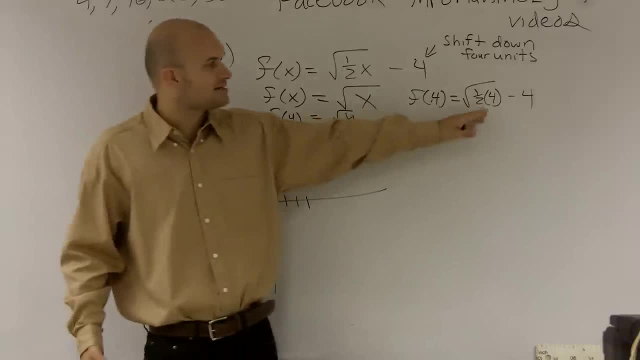 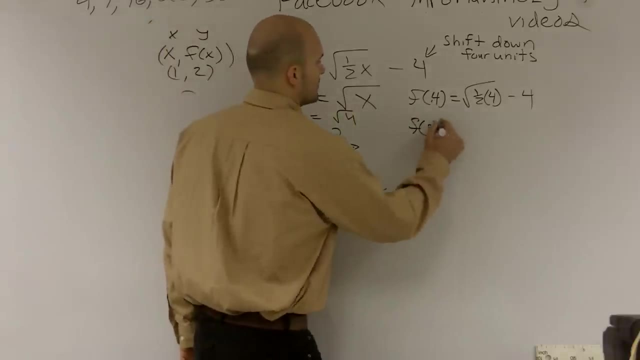 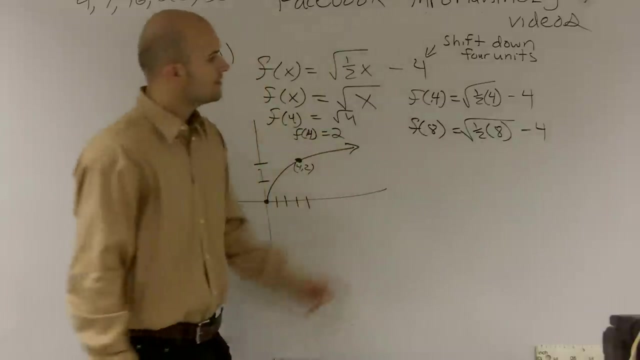 But let's pick a point, just for plain sake. Let's pick a point that actually would work on this. OK, Let's pick 8.. So let's do: f of 8 equals square root of 1 half times 8 minus 4.. 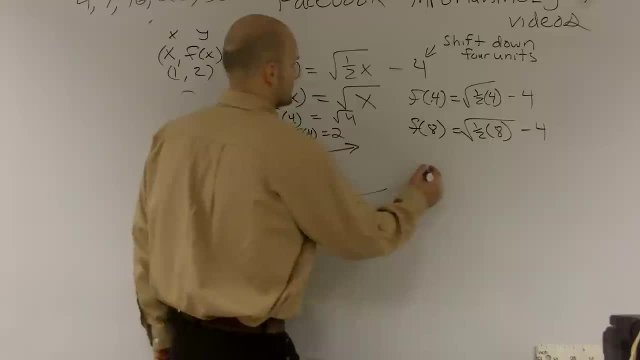 Well now, that's going to give you 4.. Square root of that is 2.. That's going to be 2.. Minus 2 is going to give you 2 minus 2.. 2 is going to be 0.. 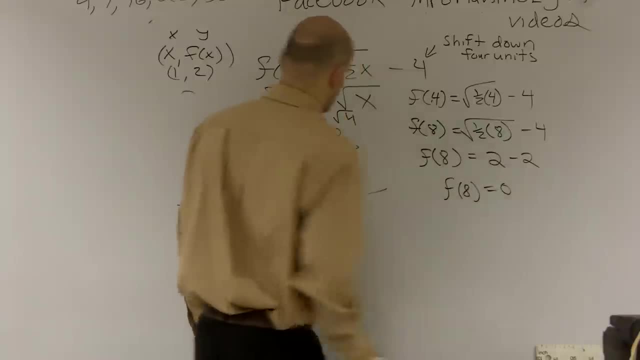 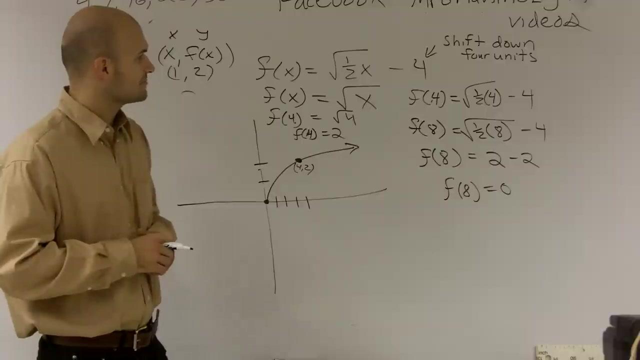 So f of 8 equals 0. And I probably should have. I didn't really want to. Let's actually hold off. I didn't really want to explain exactly that point right there, But we know that this shift- negative 4- is going to take us down negative 4.. 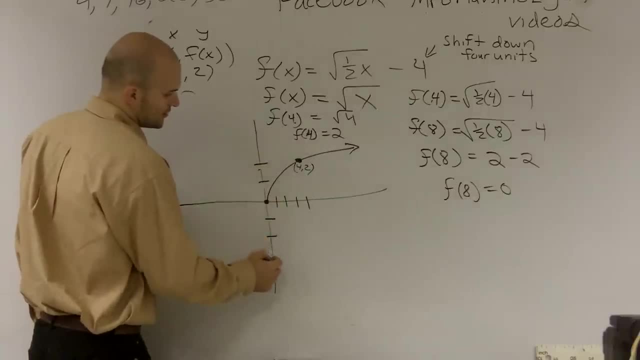 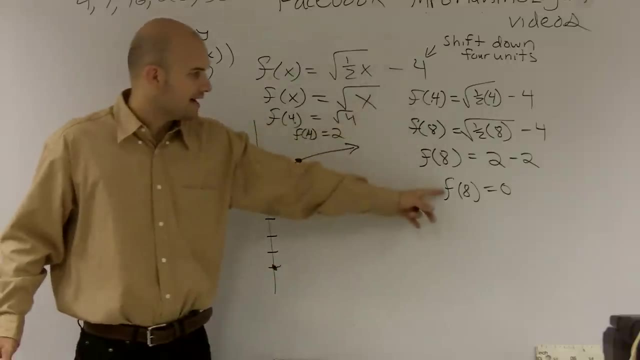 So we're going to shift this whole graph down 4.. So 1,, 2,, 3,, 4.. OK, Because it says: shift the graph down, Shift the graph down 4.. And then now my new point is: at f of 8, you get 0.. 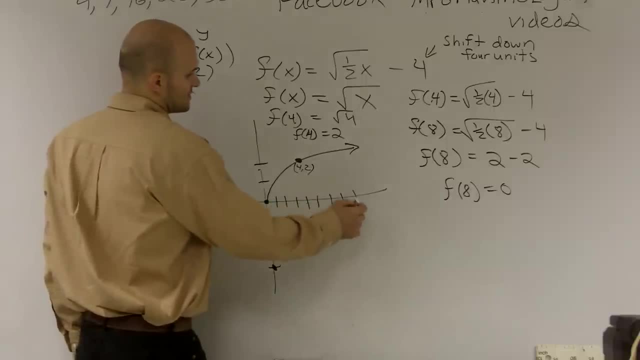 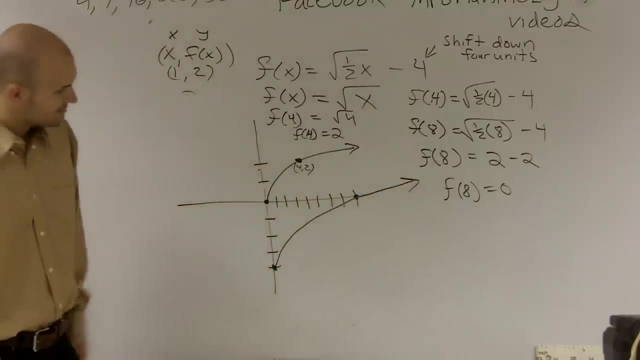 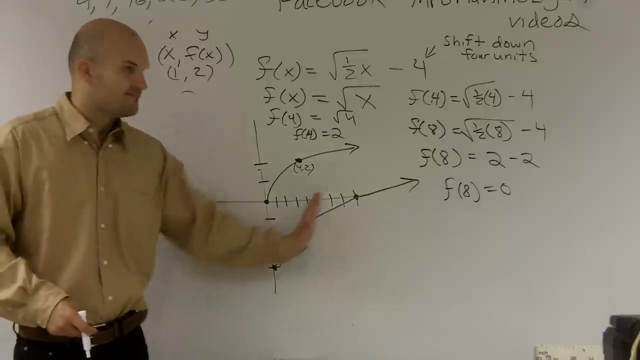 So 1,, 2,, 3,, 4,, 5,, 6,, 7,, 8.. And it's kind of hard for me to show at least a good root horizontal stretch, But hopefully you guys can see that these values are actually. 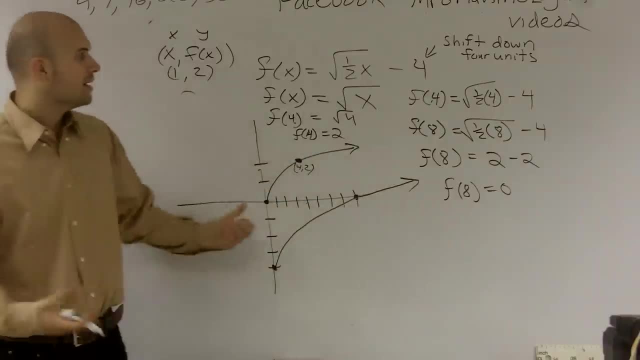 getting stretched out. OK, I know I'm not the best grapher, But OK, If you guys can just remember when you're doing this to make sure you pick values that are going to make it easy to graph, to plot. 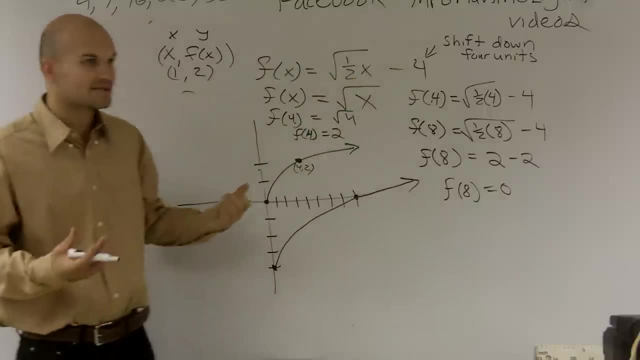 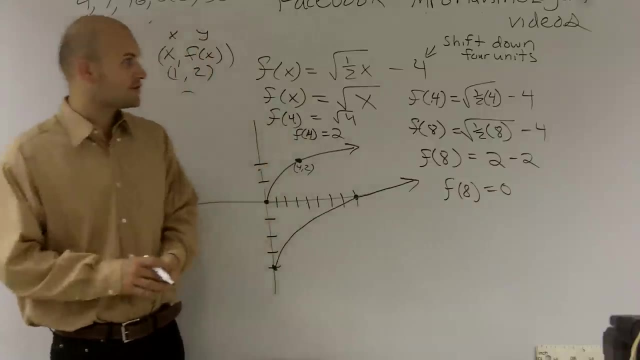 and then also just follow your shifts, everything to go and find the points. So that's how you pretty much determine if it's a horizontal stretch or a shrink, or a vertical stretch or shrink, and then how to graph it. Any questions on that?